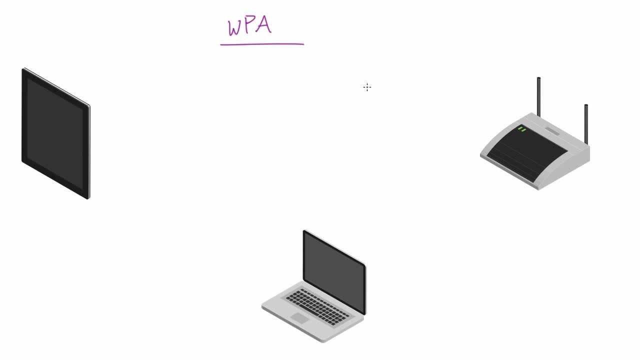 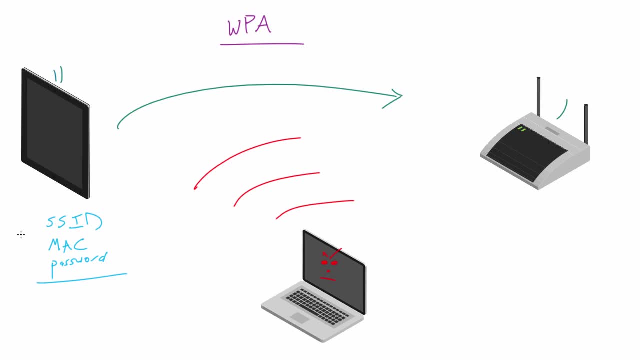 so it takes all of these pieces, runs it through a hashing algorithm and comes up with this weird answer which is like 87 JK. I'm just making this up for two explanation point. so there you go. so the reason that this actually works is because this guy right here if he knows the correct. 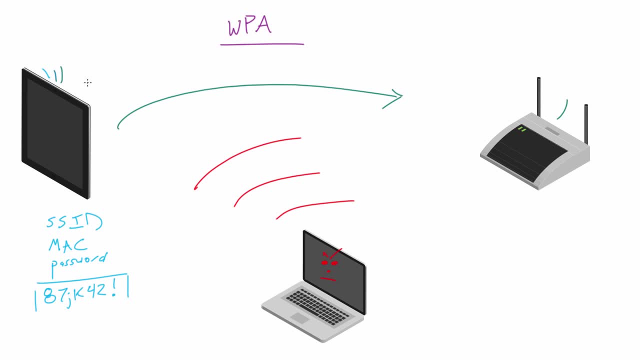 password, then he's gonna get this answer right there, so then he can get that and send it across the network. so 87 JK for two. whatever now this access point, it obviously knows the answer because it's stored in there and it knows all the other pieces, so it's gonna know that the correct answer. 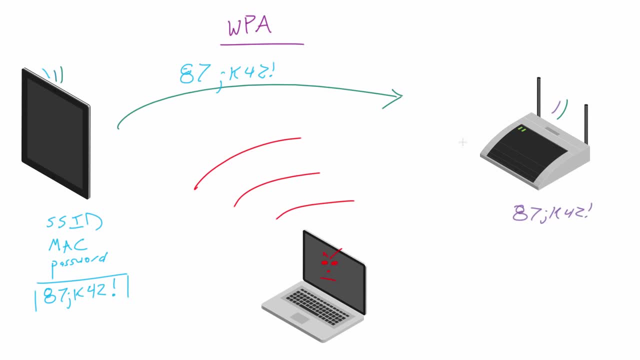 is 87 JK for two right there. so whenever it figures out the answer, sends it across the network. the routers gonna be able to check it and say, okay, this dude clearly knew the password. and the best part about this is this is how you can actually prove that you know a password without sending the actual password over. 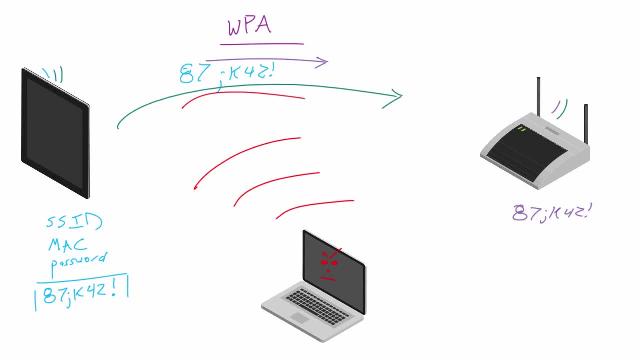 the network, so it's all actually pretty fascinating. if you want to look it up, some more highly recommend that, and this isn't, you know, all there is to it from here. they do other stuff, like make their encryption key and once they both have the encryption key, that is how this tablet and this access point can encrypt. 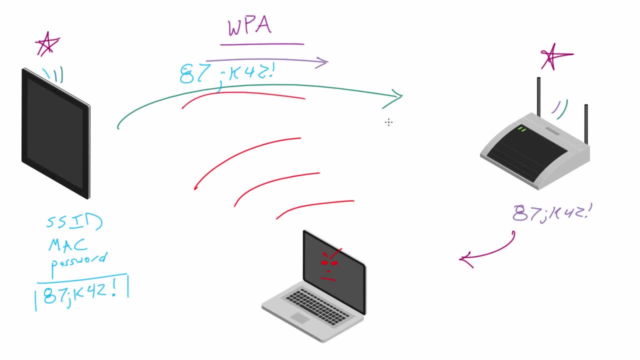 in decrypt packets for a nice, secure conversation and, if you remember, a couple tutorials ago, whenever we view those packets and we were trying to read them, it looked like all mumbo-jumbo. well, the reason for that is because it was encrypted using the encryption key that was derived from, basically, this: 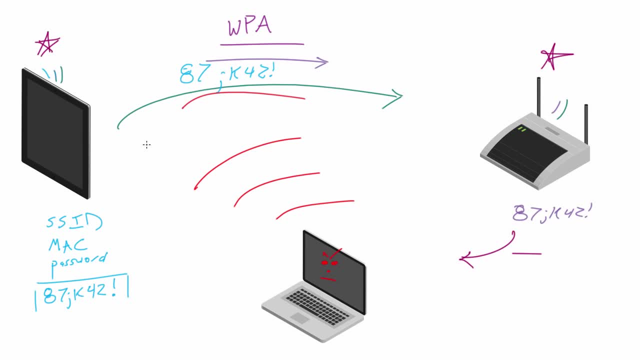 authentication method, known as a four-way handshake. so this is all pretty technical and, like I said, we really don't need to understand most of this. what you really need to understand is this: if you can figure out all the pieces to the puzzle, then you can basically figure out everything else. in other words, once you 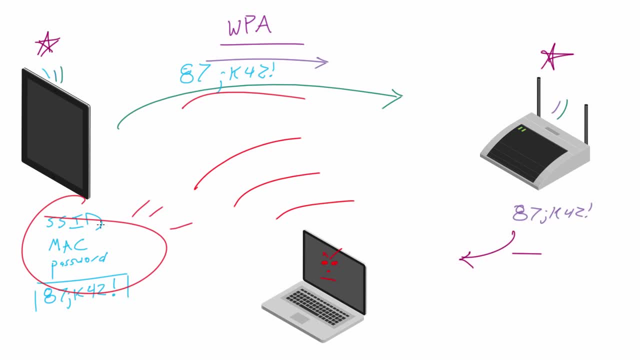 know the pieces that go into making up the keys, then what you can do is not only can you join the network yourself, but you can decrypt everyone else's data that's on the network. all right, that's pretty cool, but the problem is that we don't have these pieces specifically. we are missing the password. 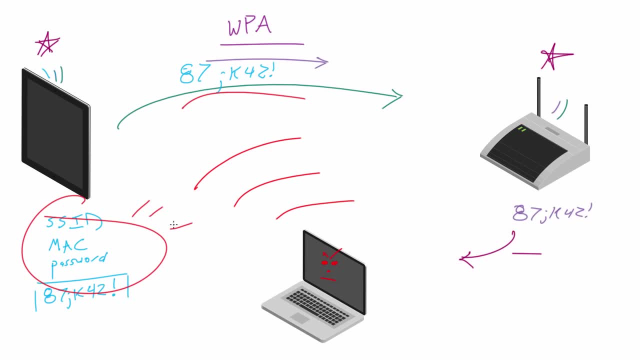 so we don't have these pieces specifically, we are missing the password. so, you know, I guess that's it, I guess we'll go home. oh, wait, a second, let's think about this. I mean, we may not have the password yet, but what information do we have? what we have, the entire formula, I mean all the 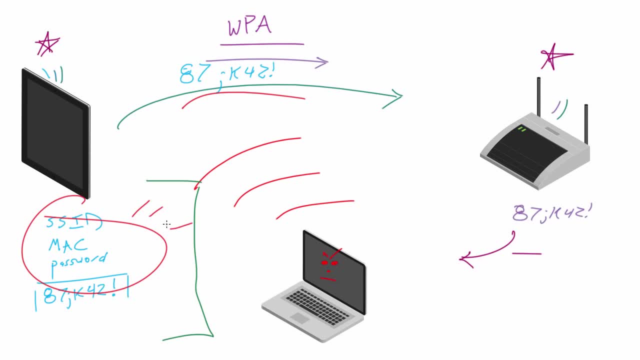 pieces to the formula. but we know how the formula works and we also have some other critical pieces that we may need. I mean we can see the answer in plain text, no problem. you may think that that's worthless, but I mean we can get the SSID, we can get the MAC and all of the other pieces except from the. 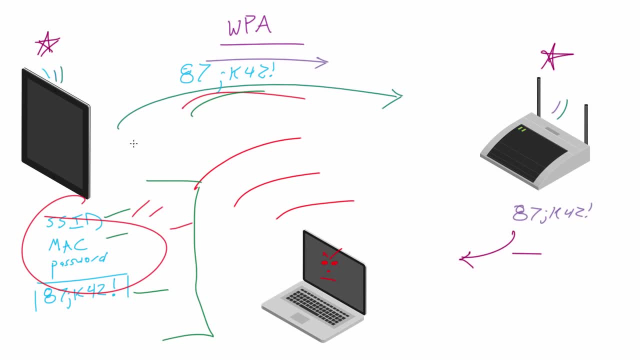 password we can just pull out of plain text. Alright, so we have all these pieces, but the only thing we're missing is this. So what we can do from here is actually really cool. We can have a huge list of passwords and we can just start plugging them in for this part of the puzzle.